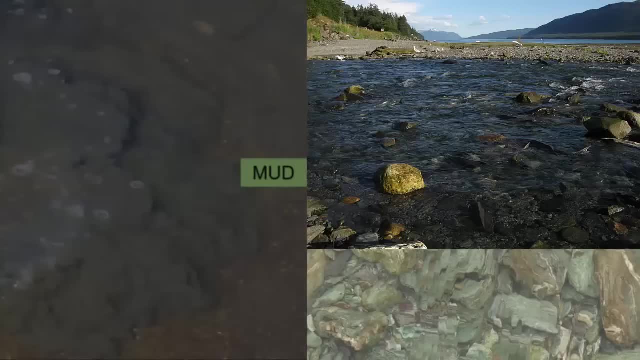 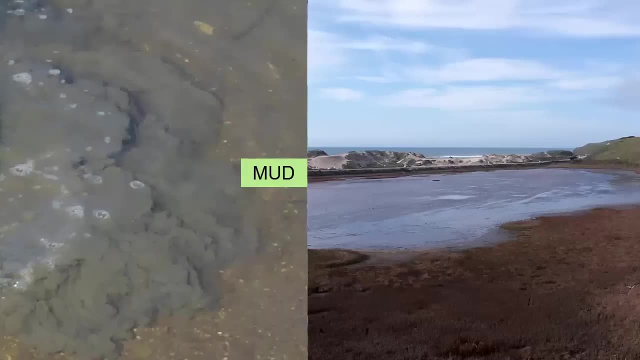 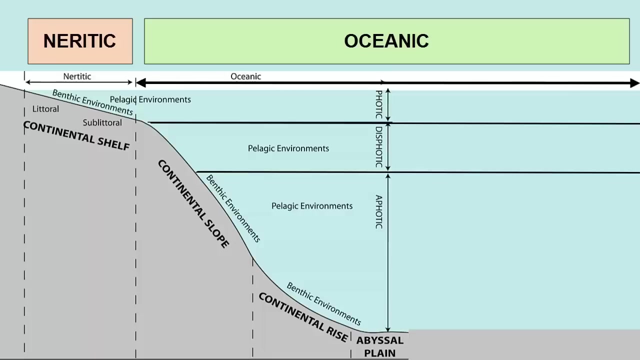 sizes found in the ocean. The largest grains, the heaviest, settle quickly in still water and require high-energy water to be picked up and carried. The smallest grains require perfectly still unmoving water to settle out. Ocean environments are separated into two. 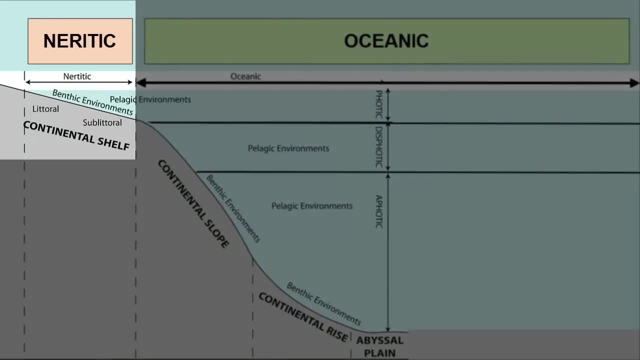 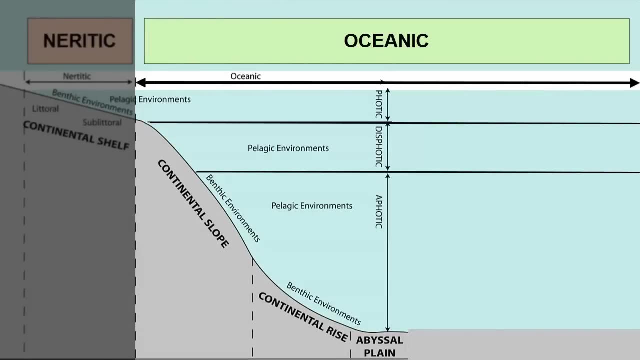 major geographic zones: Neuritic over the continental shelf and oceanic over the slope rise, abyssal plains, mid-ocean ridges and trenches. Neuritic waters tend to have faster moving currents, interacting with surface waters in the 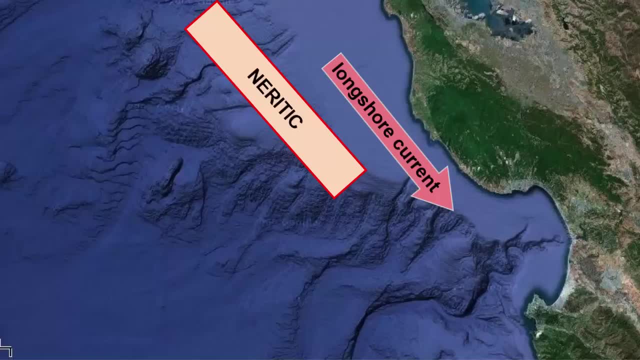 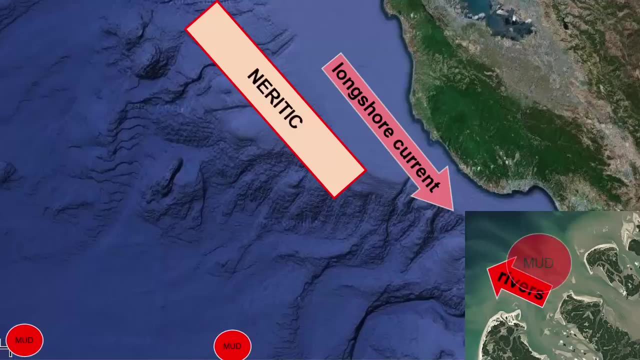 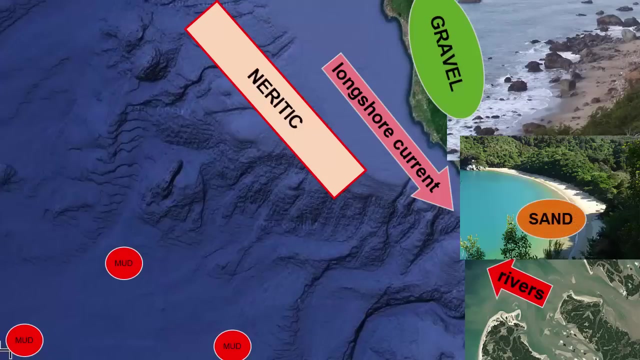 shallow bottom. These waters can pick up and shift around larger sediment grains. Rivers that enter here will retain mud-sized sediment in suspension and can carry them quite a distance. offshore Gravels tend to stick close to shore. Fine sands collect in medium-energy coves and can be carried. 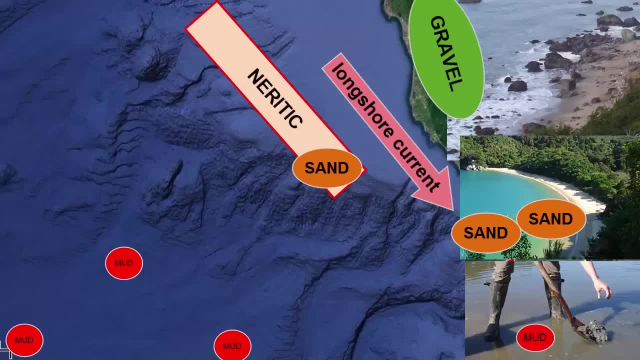 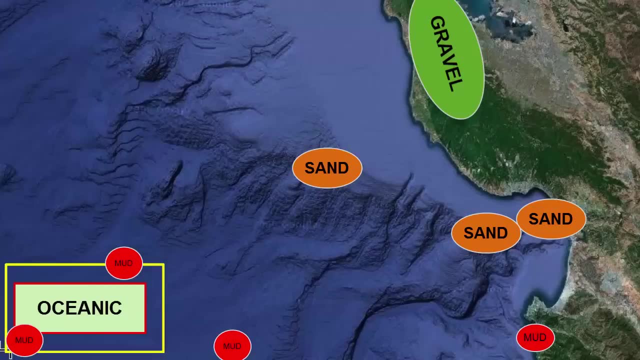 out to the edge of the shelf. Muds settle out only in closed off, no energy lagoons. Oceanic waters are deep with no currents that touch the bottom. Gravels and sands cannot be transported out here by anything other than floating. 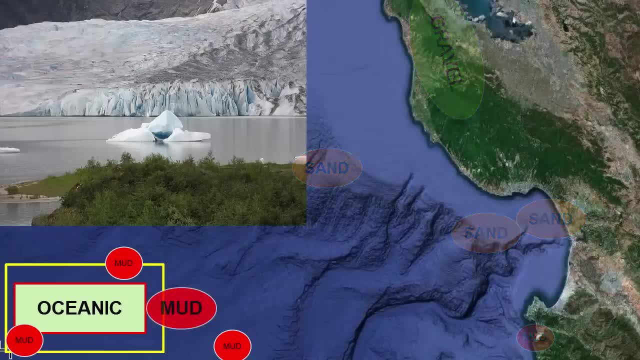 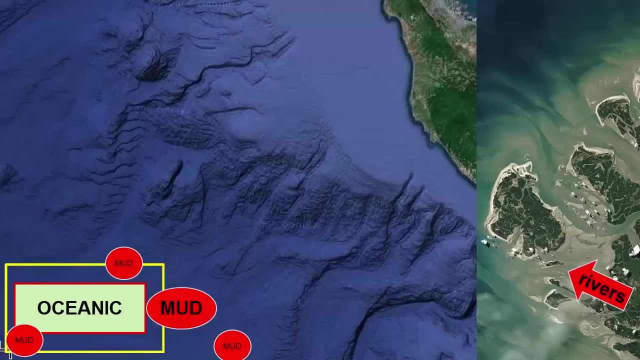 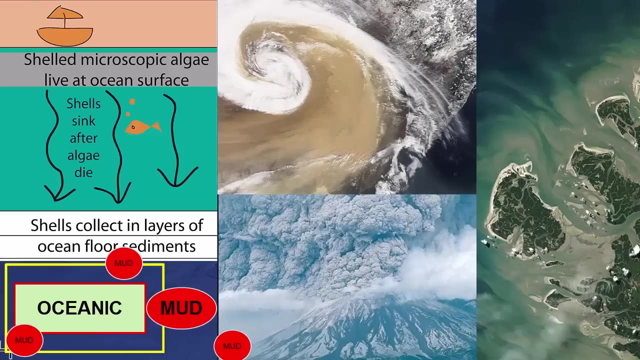 icebergs. so the sediment that falls here is only the muds. Where do these muds come from that get out to the oceanic zone? Nearby rivers that have a lot of suspended sediment, airborne dust and ash that settles on the surface and the shells and debris of organisms that live in the? 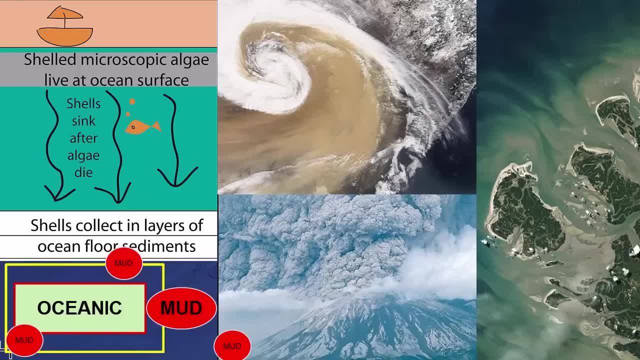 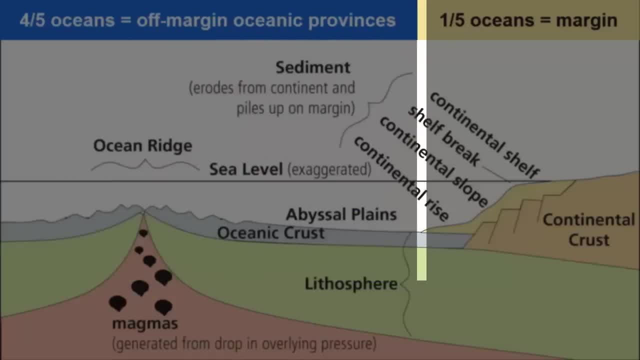 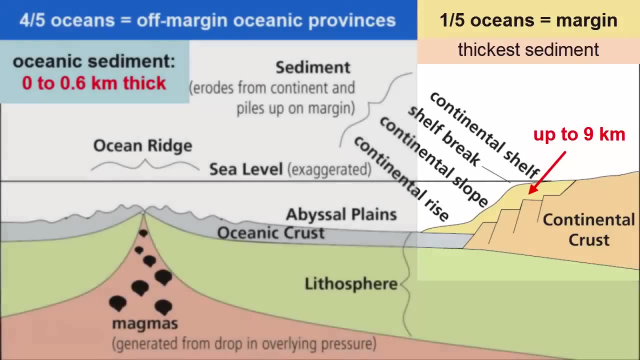 surface waters and settle to the seafloor when those organisms die. The oceanic zone represents four-fifths of the world's ocean environments. However, the sediment that collects in the margin environment is the thickest in the world, up to nine kilometers thick compared with the oceanic sediment thickness. 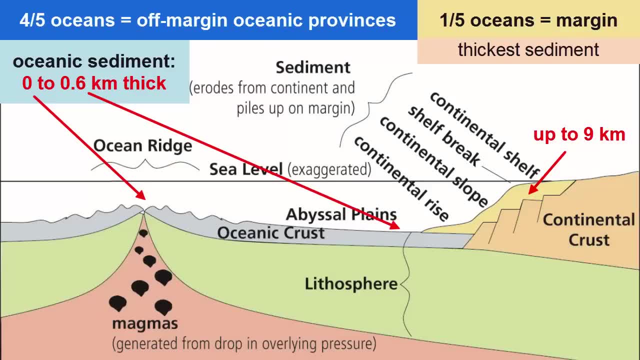 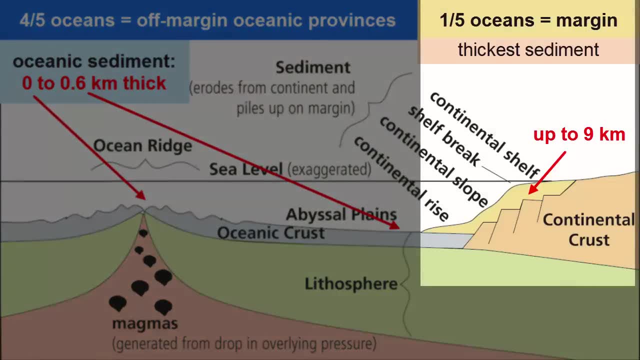 which increases from zero at the ridges to 0.6 kilometers at the thickest oldest edges of the abyssal plains. Even though the sediment that collects in the margin environment represents only one-fifth the ocean's surface, its sediment volume represents almost 90% of the total ocean sediment. 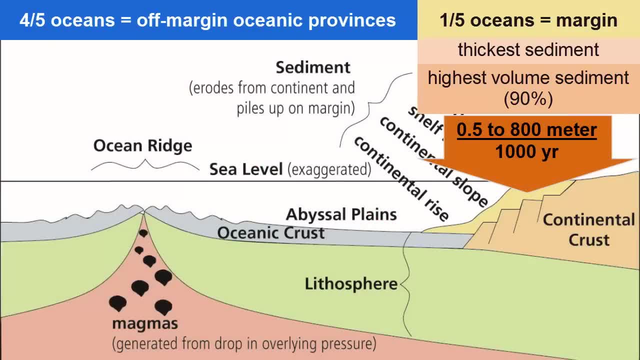 Why Sediment collects here much faster, at rates from a half to 역, straightforward 800 meters per 1,000 years. For comparison, in the oceanic zone sediment collects at its fastest one centimeter per thousand years. Pause now. 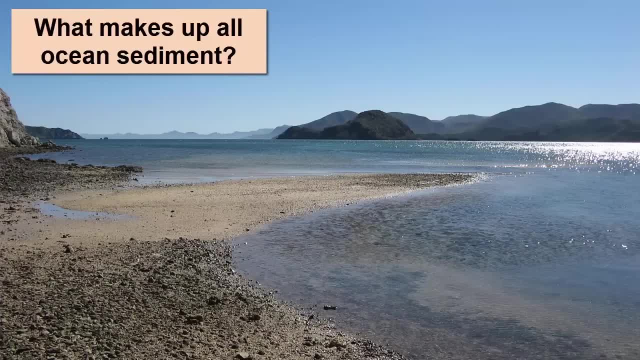 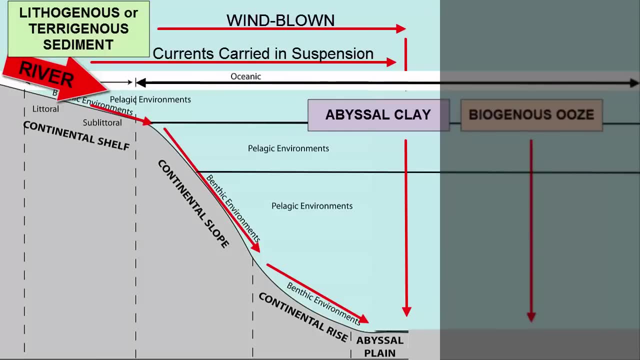 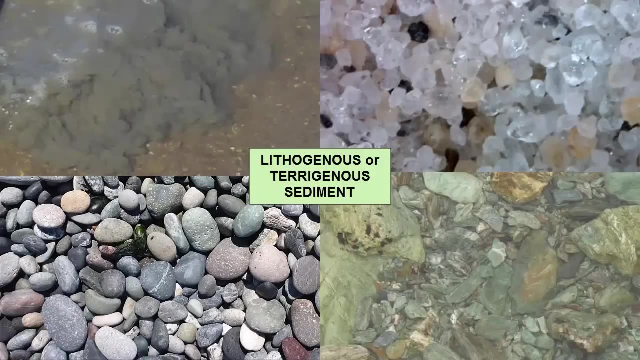 What makes up all these sediments? There are four major sources of sediment to the ocean and of course, each gets its own name. We call sediment that originated from rock weathering on land lithogenous or terigenous sediment. What is it made of? Bits of rocks and minerals? 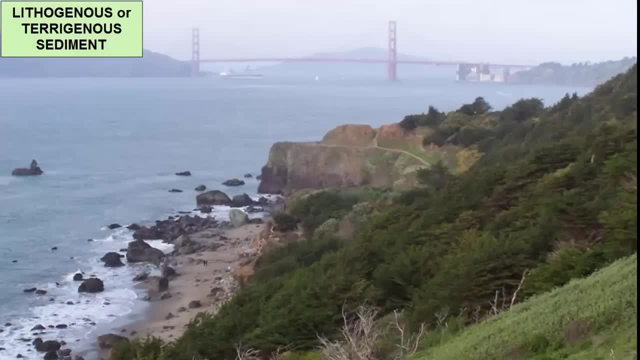 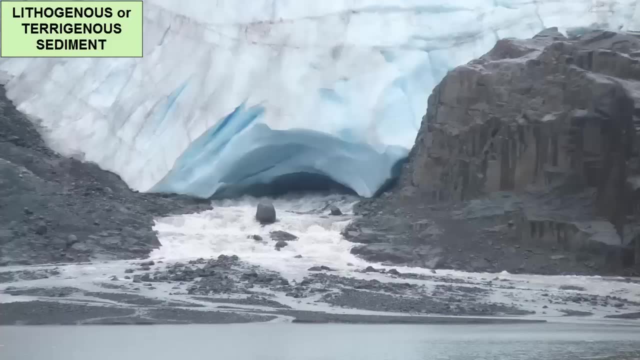 When, next to a weathering cliff, like along an eroding coastline, the material is made of bits of the rock in the cliff and gravity carries them towards the ocean. When dropped by glaciers, these sediments can be quite large and come relatively preserved from the backcountry. 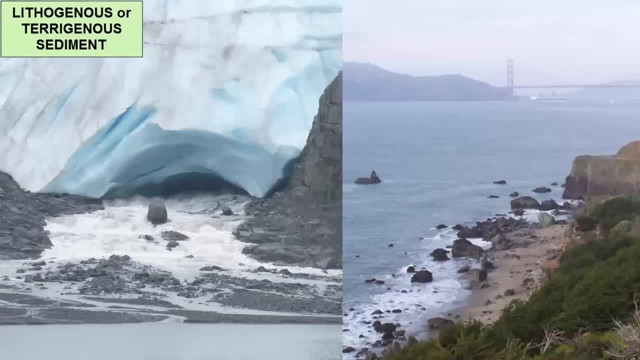 far and wide. When you're in a situation where the sediment is quite large, you can get some inland. We call both of these types of sediments immature because they haven't been modified much by travel. They can be angular and poorly sorted, consisting of: 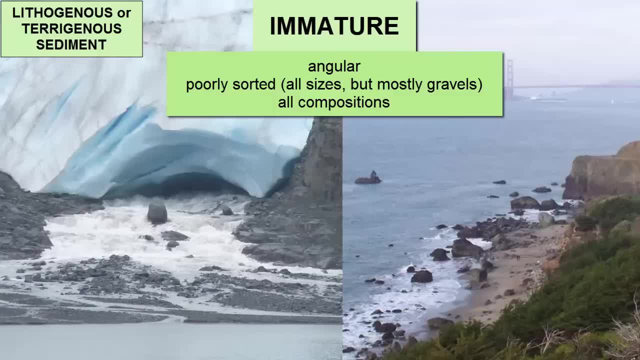 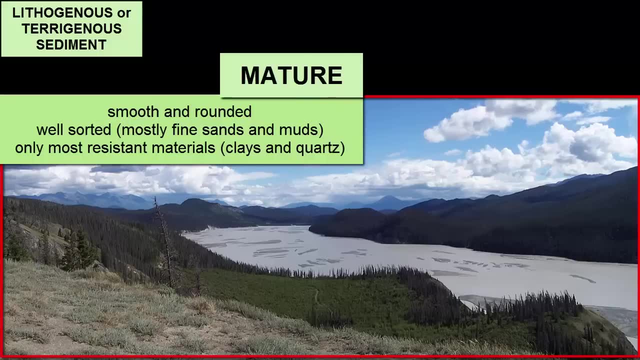 grains of all compositions, shapes and sizes, mostly gravels. When lithogenous sediment is carried by rivers, on the other hand, it becomes mature Grains, decrease in size to fine sands and muds. Why, During transit, the grains are. 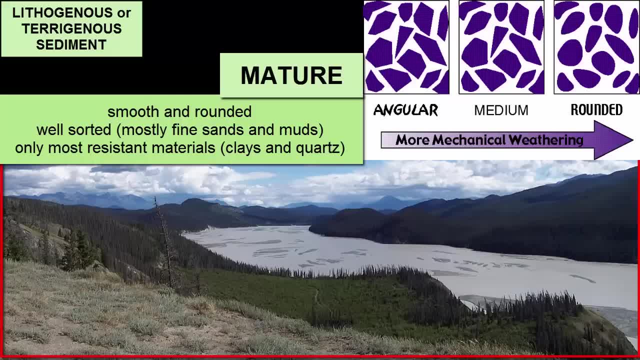 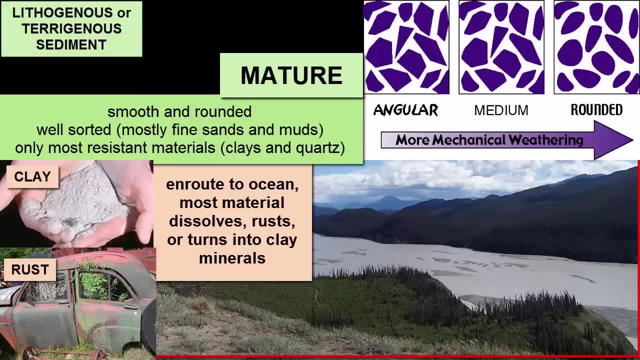 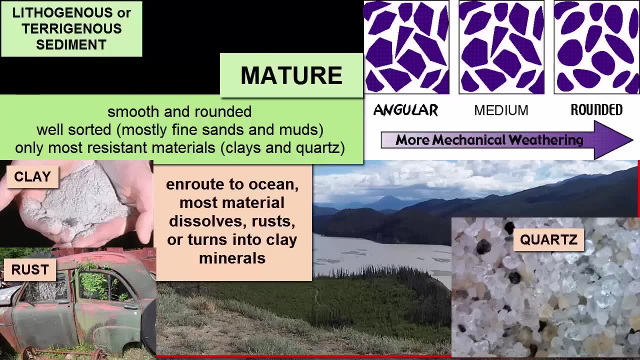 knocked around and hit each other, They physically break down into smaller pieces. They also break down chemically. Most of the material dissolves or is turned into clays and rust. The most resistant materials, predominantly quartz grains, which don't dissolve or turn into clay or rust, remain. 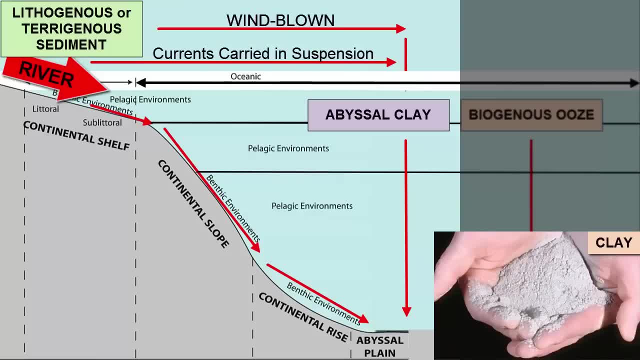 Clay minerals are mud-sized and are the most common byproducts of rock weathering on Earth's surface. Some of these clay minerals make it out to the oceanic zones, either by sea or by sea By being held in suspension near large river deltas or by being carried by winds off desert. 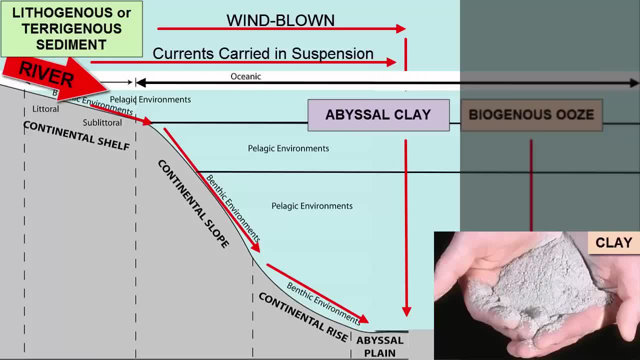 and mountain areas. We call those clays abyssal clays as they are found in abyssal plains. We'll return to them shortly, As lithogenous sediment dominates the coastal margins and accumulates at the fastest rates of all sediments there and also reaches out. 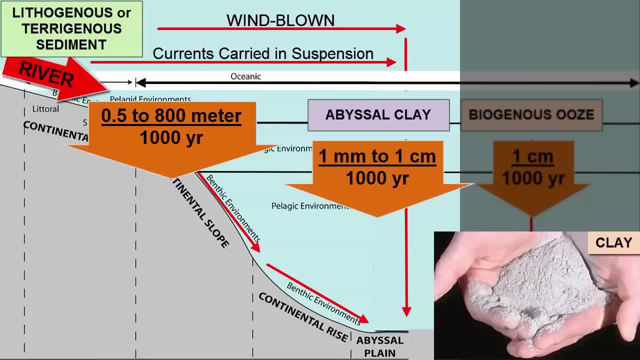 in its mud-sized form to the deeper parts of the oceans, predominantly as abyssal clay. lithogenous sediments make up the largest percentage by volume of the ocean's surface. However, because most of this volume stays close to the margins and piles up there thickly, 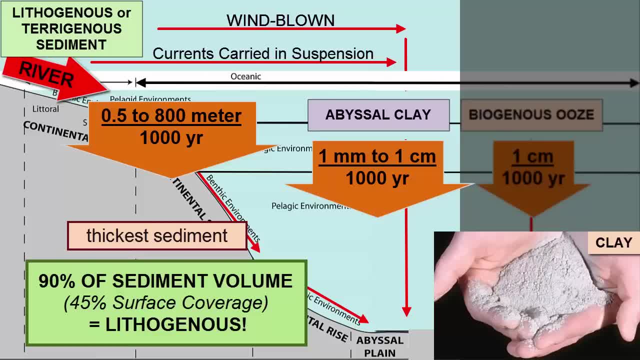 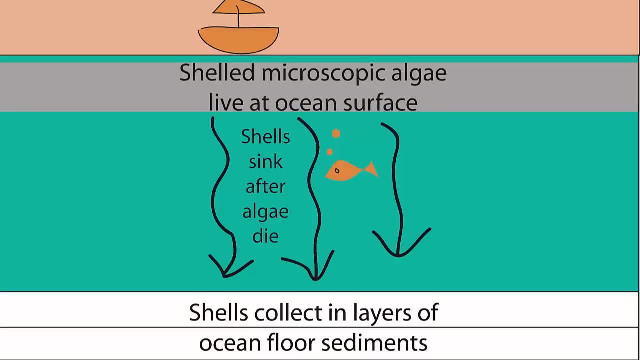 they represent only 45% of the total seafloor surface coverage. The sediment that covers most of the seafloor surface is biogenous, which consists of shells of dead organisms and dominates the oceanic zones. The most important contributors to biogenous sediment are the single-celled autotrophic. 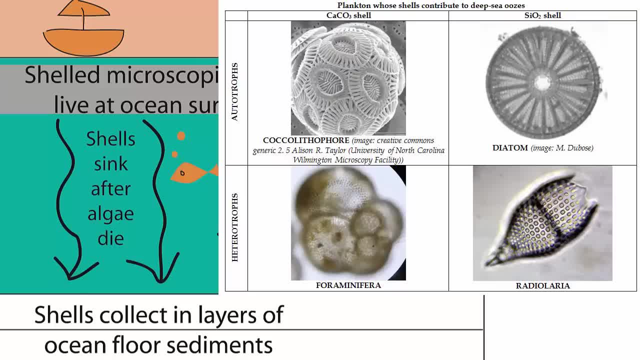 and heterotrophic plankton. They live in the surface waters. Billions of these organisms live and die, with lifetimes of days to weeks. Their shells collect on the bottom of the seafloor and contribute to siliceous and calcareous oozes, depending upon whether the shells are made of silica. 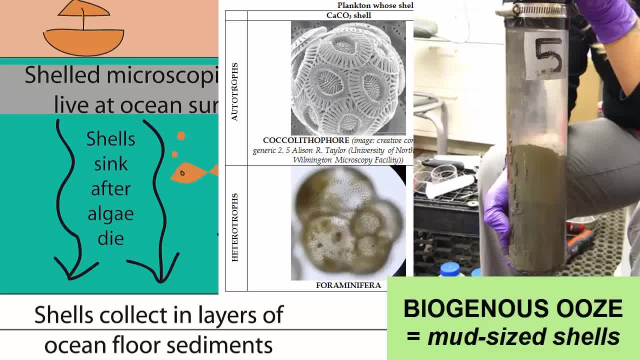 or calcium carbonate. The term ooze tells us a lot about the consistency of these sediments. They are all mud-sized, a very fine flower-like material. Larger, gravel-sized sediments are made of silica or calcium carbonate, or calcareous. 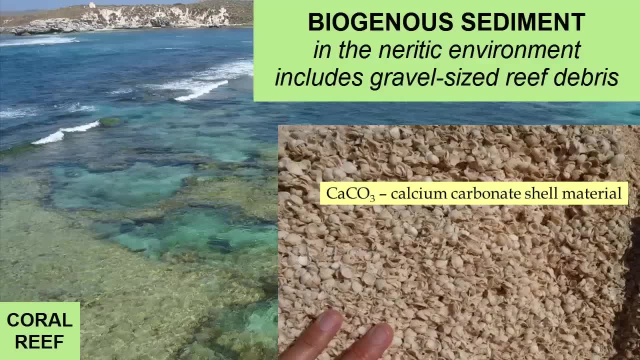 oozes. The term ooze tells us a lot about the consistency of these sediments. They are made of silica or calcium carbonate or calcium carbonate. The serine-type bite shells contribute to neuritic nearshore sediments where there are. 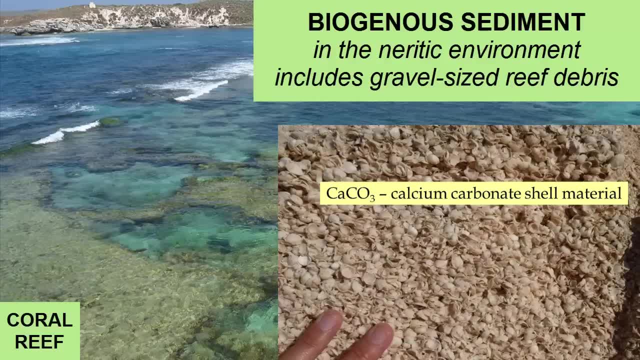 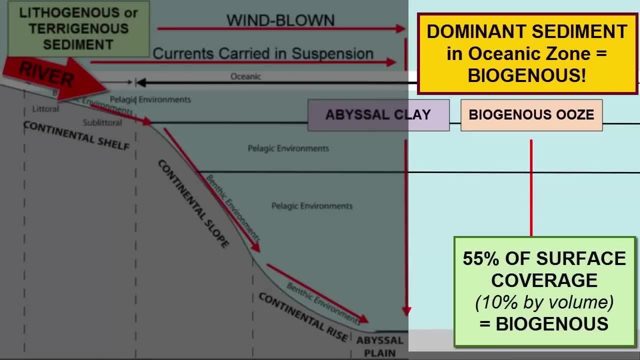 large reefs, either tropical coral reefs or cold-water reefs made of molluscs like mussels and limpets. We'll return to the oceanic oozes shortly to describe them in more detail. Another type of sediment called hydrogenous represents minerals that are produced from. 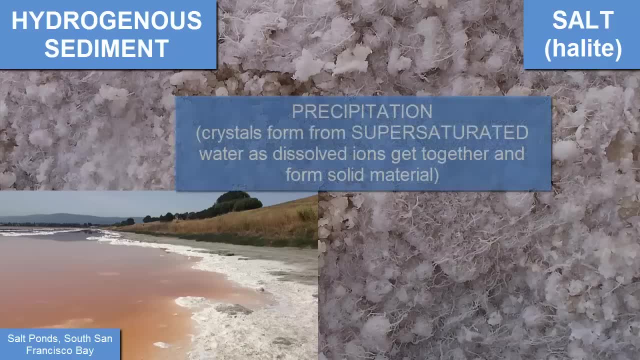 ions that were originally dissolved in water. We call that process precipitation. Seawater has many dissolved ions in it And in numerous locations those ions are called hydrolysis. Hydrogenous sediment is a sediment from the ocean's surface or the ocean's surface. 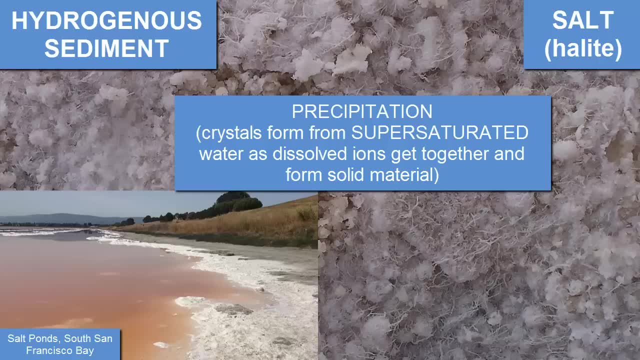 which is the surface of major rivers. It is a sediment of coverage In the wetlands, and those ions reach a concentration that is higher than can be dissolved by the water anymore, either because of evaporation of water or because of an influx of dissolved ions. 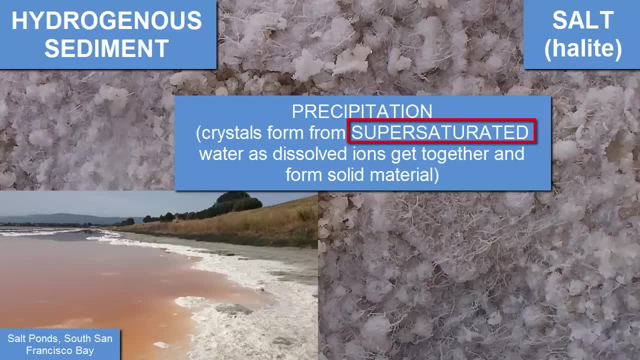 We call that state supersaturated, and you can learn more about this in the seawater chemistry video tutorials. For now, we'll focus on where to find these precipitated hydrogenous sediments At shallow inland seas, where rains are limited and evaporation rates are high. minerals can 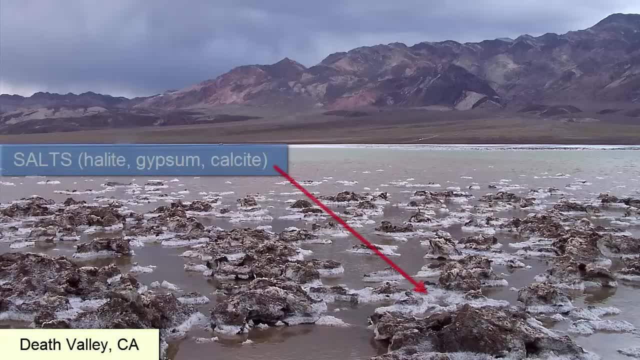 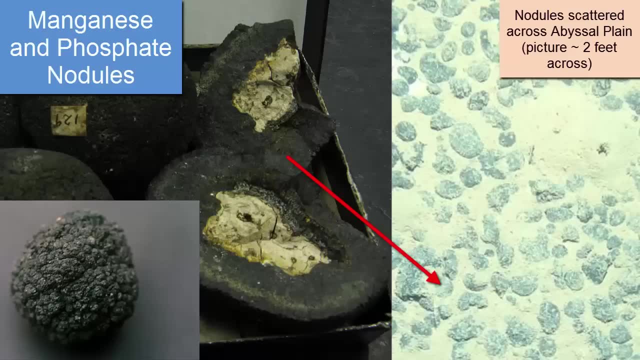 precipitate in high amounts. These minerals consist of halite, table salt, gypsum, drywall material and calcite. In some areas of the abyssal plains, dissolved phosphates and manganese become supersaturated and precipitate as nodules that grow bigger over time as new material precipitates atop. 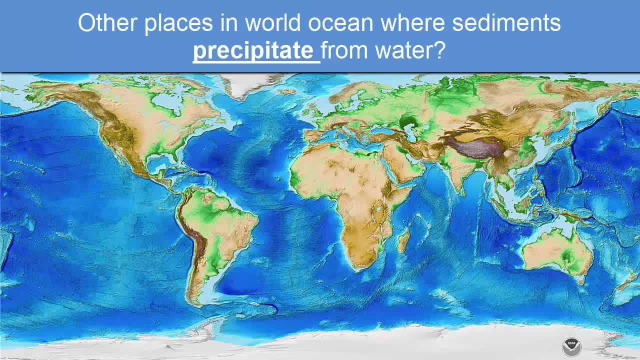 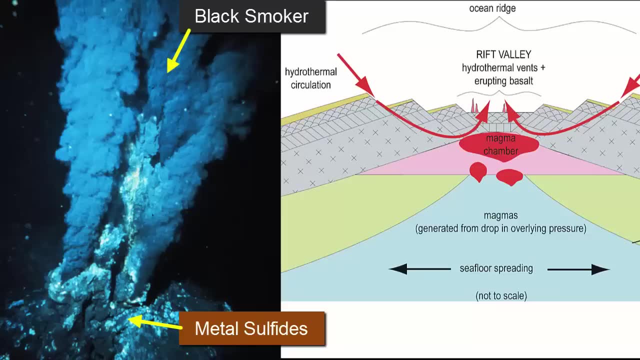 the older material, Any other place in the ocean where sediment precipitates from solution, Something we discussed in the plate, tectonics and earth formation. video tutorials. Hydrothermal vents, Hot waters rich in sodium, Hydrogen-dissolved ions leached from the ocean crust enter the colder seawater. 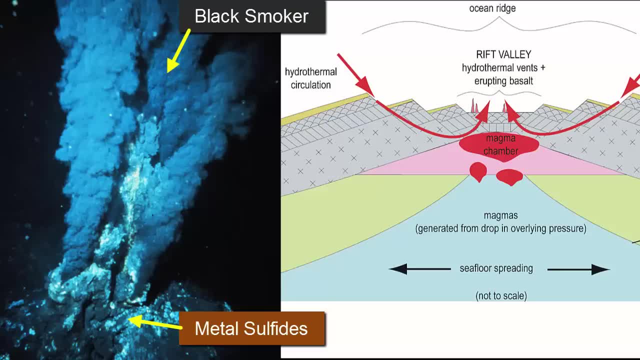 As that hot water cools, it becomes supersaturated with dissolved ions. Cold water can dissolve less than warm water. That's why, when cooking, we heat up our water when we want to dissolve things like sugar or salt in it. Hydrogenous sediments are found in many places across the oceans, but they represent less. 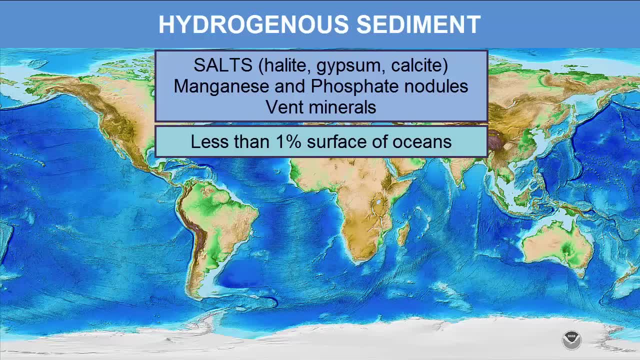 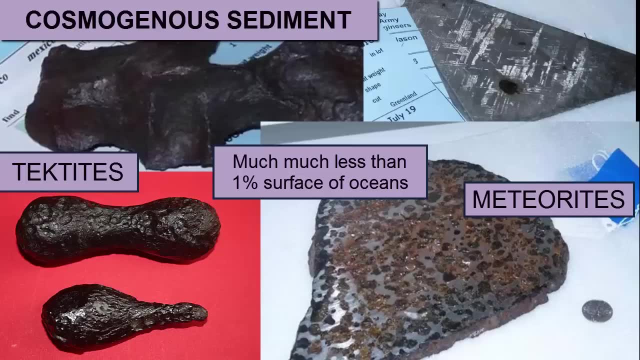 than 1% of the surface area, as they are largely scattered. The most uncommon sediment found in the ocean, but still famous, is hydrogen. The most common sediment found in the ocean, but still found in abundances greater than on land, is cosmogonous sediment, meteorites that fall from space and tektites which 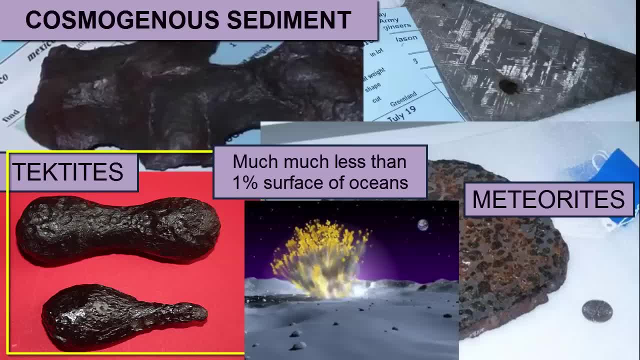 are bits of earth's crust that have been ejected into space after a meteorite impact excavates a crater. This ejected, excavated crustal material melts as it exits the atmosphere and solidifies as it falls back down, producing a spherical, teardrop-shaped glass nodule with eroded pits. 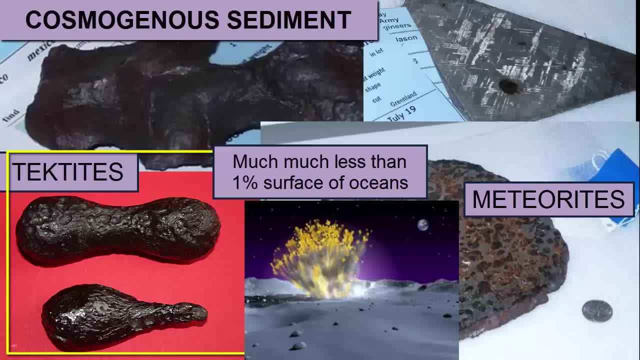 created by its journey back down through the atmosphere. The most common sediment found in the ocean, but still found in abundances greater than on land, is cosmogonous sediment meteorites that fall from space, as they are largely scattered across the ocean. The most common sediment found in the ocean, but still found in abundances greater than on land, is cosmogonous sediment: meteorites that fall from space, and tektites, which are bits of earth's crust that have been ejected into space after a meteorite impact. 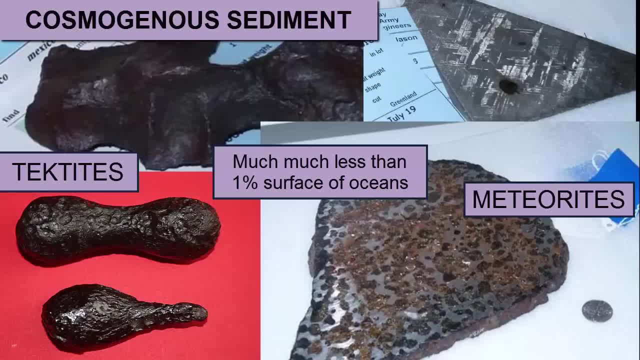 Why are these found in the oceans in more abundance than on land? Simply because of the slow sedimentation rate of the oceans, Where sediment collects at rates as low as 1 centimeter per 1,000 years, it's easier to find the tektites and meteorites that fall among them. 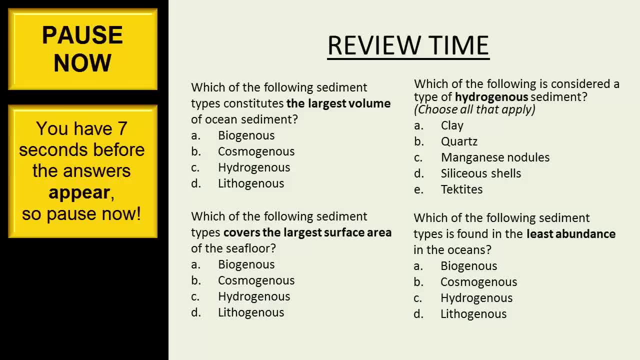 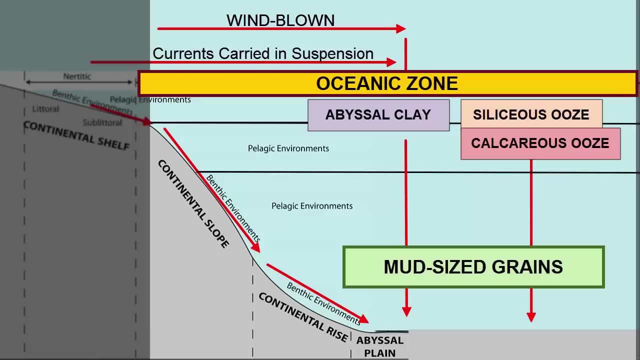 Pause now. Now let's return to the oceanic zone and look more closely at the mud-sized abyssal clays and siliceous and calcareous oozes that form. there Are all three found in the same location. In most cases, one is the dominant. 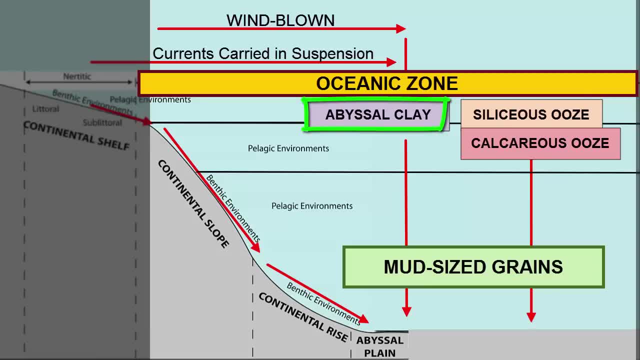 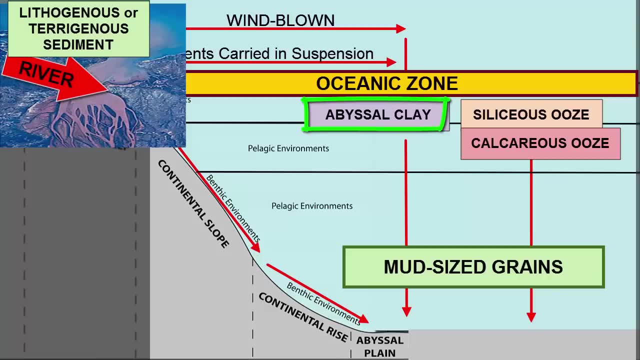 Why? Abyssal clays, remember, are lithogenous or pterygianous, so they will dominate near high-volume rivers with large deltas, Without rivers nearby. abyssal clays come from the settling of airborne dust and ash that's been blown from the land. 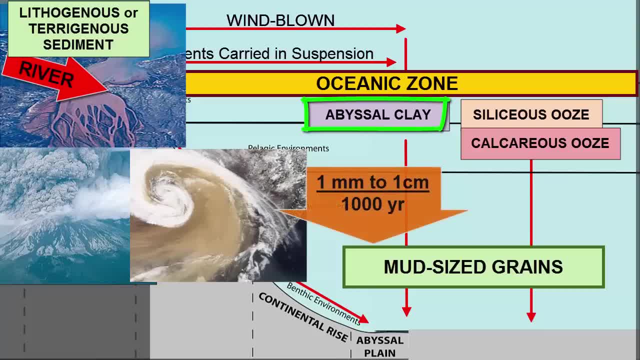 If there are nearby deserts with high wind activity, the rates of abyssal clay settling can be comparable to that of calcareous or siliceous shells. So the settling rate of abyssal clays in the deep oceans can be anywhere from one millimeter. 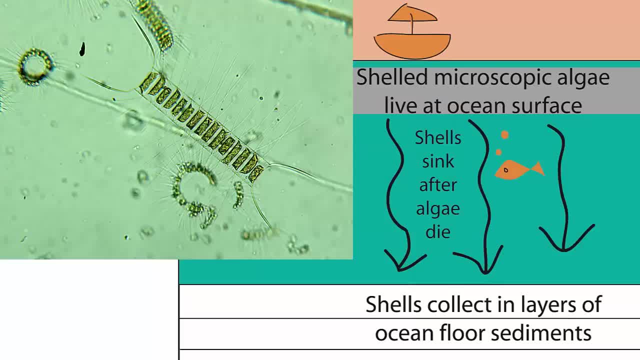 to one centimeter per 1,000 years. We call the organisms that live in the surface waters plankton. free-floating can't swim faster than currents. If they are autotrophic, make their own food. They are the bottom of the food chain and are referred to as phytoplankton. 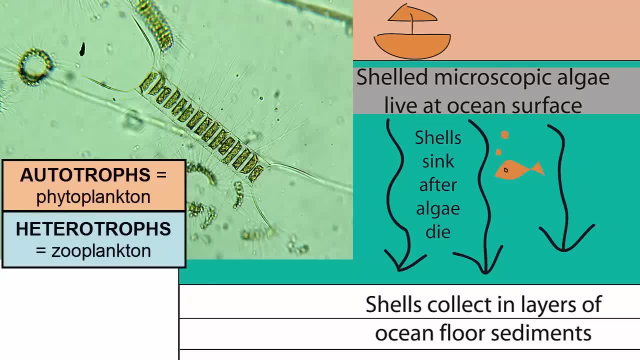 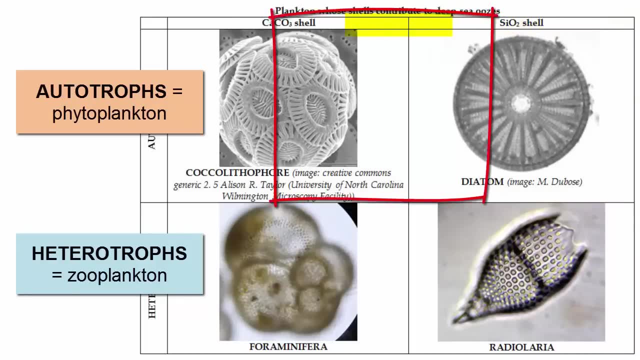 Heterotrophic plankton are referred to as zooplankton. Diatoms are phytoplankton with silica shells. Cocolithophores are phytoplankton with calcium carbonate shells Radial area are the most common zooplankton with SiO2 or silica shells. 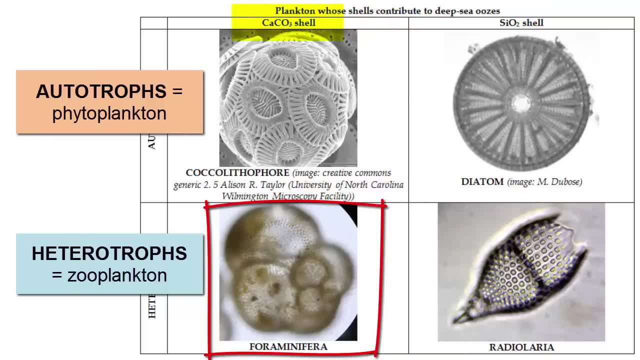 Foraminifera are the most common, with calcium carbonate shells. These four organisms play very important roles in the world's oceans and it's valuable to memorize these names and shell types now, as they will appear many times throughout future video tutorials. 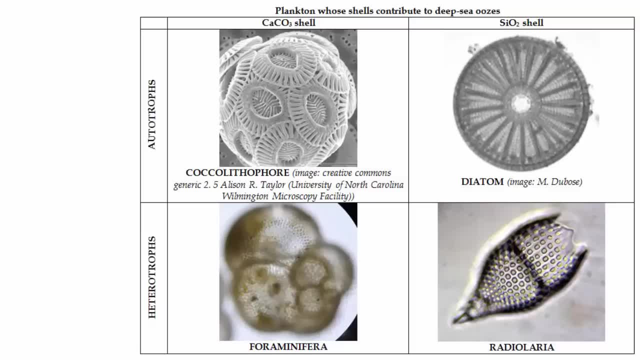 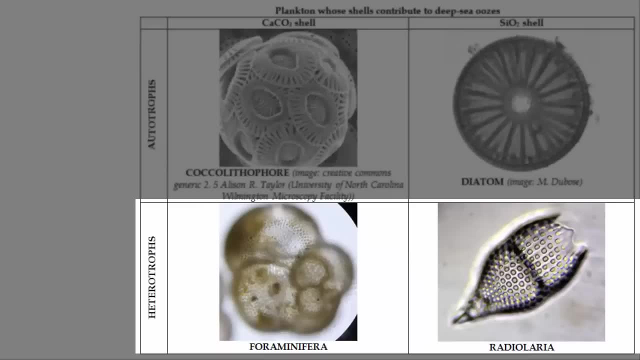 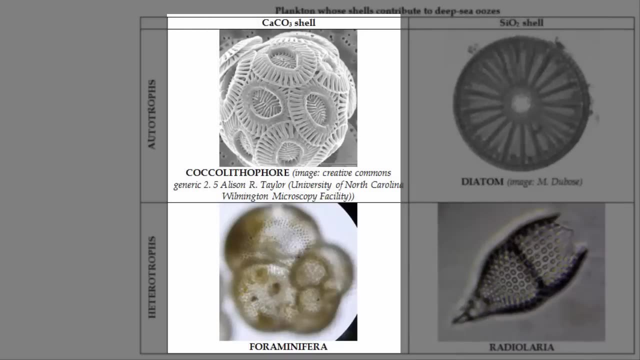 We'll review one more time. then you'll take a quiz. Diatoms and cocolithophores, Radial area and foraminifera. Silica shells, Diatoms and radial area, Calcareous shells, Cocolithophores and foraminifera. 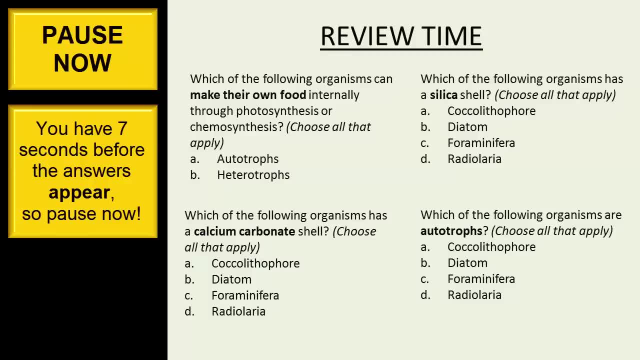 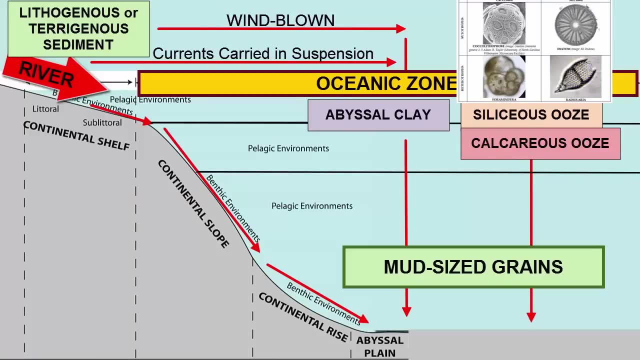 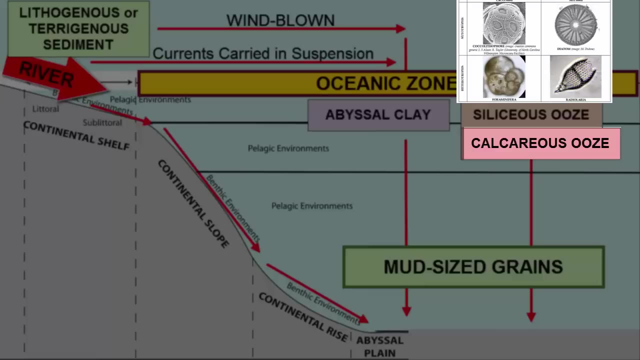 Pause now. So where do these organisms thrive, and hence their shells dominate? the oceanic muds on the seafloor. Calcareous shelled creatures are the most abundant organisms in the world's oceans, so theoretically, their shells should dominate all deep sea muds. 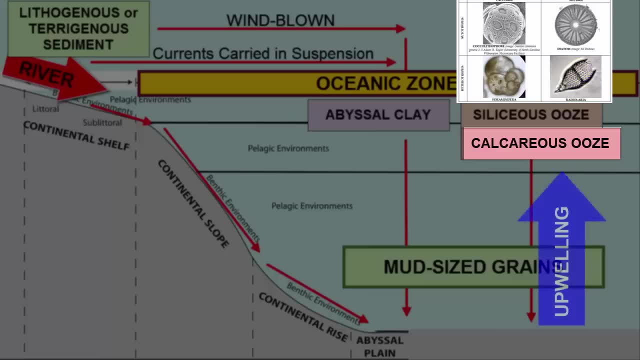 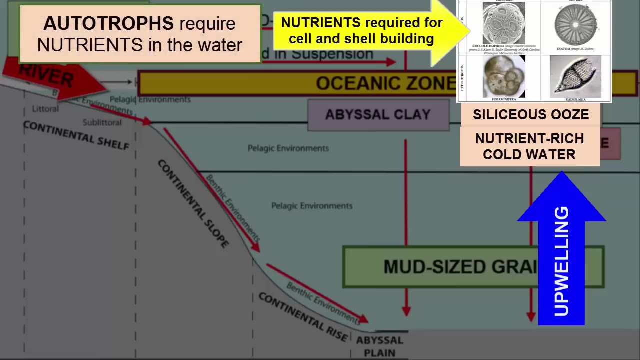 That would be true except for two things. First, in areas where deep water rises to the surface, a process called upwelling silica shelled organisms thrive. These waters are cold and filled with nutrients. Nutrients are dissolved ions that autotrophs pull from the water to use for building cells. 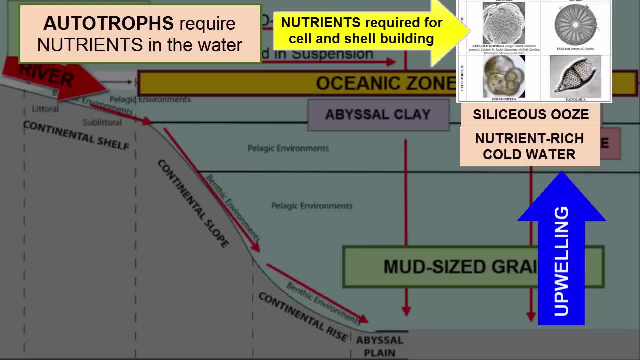 and shell material. All autotrophs require that the water have nutrients. Heterotrophs get their cell-building and shell-building nutrients from their food. So what does that mean? It means that the water has nutrients. Since autotrophs make their own food, they need to get their nutrients from the surrounding. 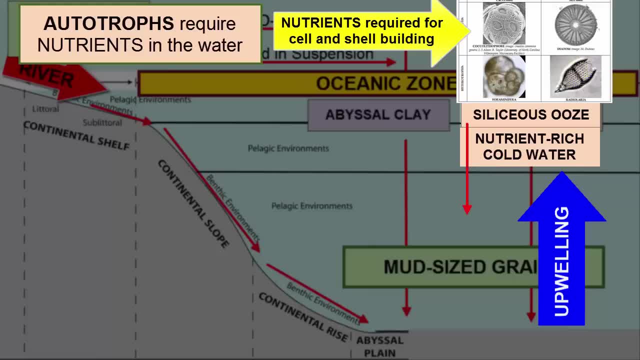 water. Silica shelled autotrophs are adapted to cold, nutrient-rich water, while calcareous shelled autotrophs tend to prefer warmer waters and don't require as high a nutrient content. So siliceous oozes dominate under areas of upwelling. 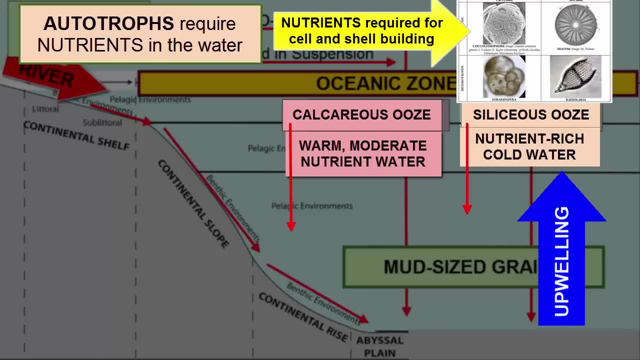 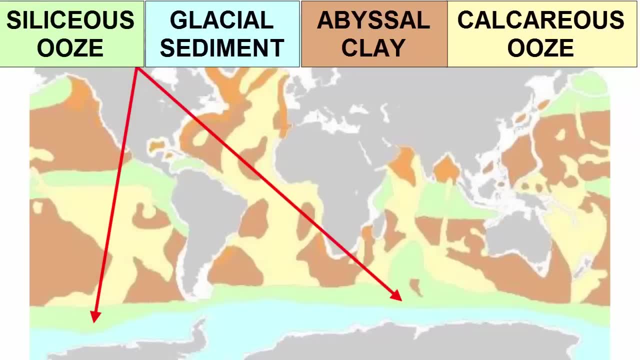 Though some calcareous shells might also be found in these oozes, along with abyssal clays, the siliceous shells dominate. Where are these areas? Upwelling can occur anywhere at any time, but it is typically found year-round in the 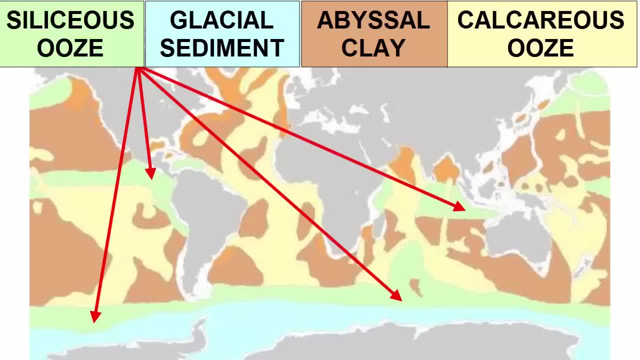 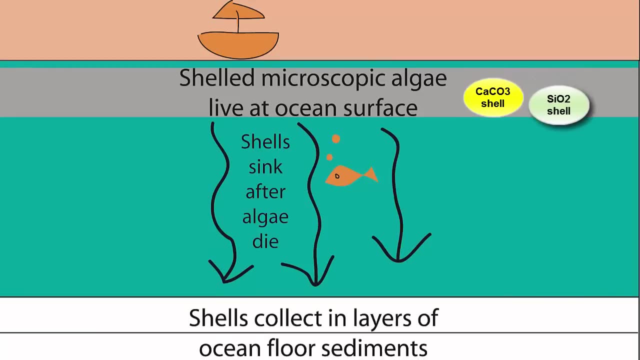 waters surrounding Antarctica and along the eastern edges of the ocean basins along the equator. We'll learn more about why that's true in the video tutorials that deal with ocean currents. So everywhere else there should be calcareous oozes, Not quite. 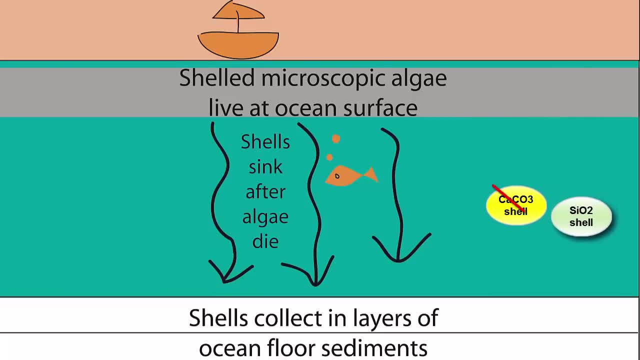 There's one remaining issue to take into account. Calcareous shells will dissolve in acidic waters And as water gets deep, cold temperatures and high pressure mean more carbon dioxide is dissolved. More carbon dioxide means more acidic. For more information, refer to the video tutorial on carbonated oceans. 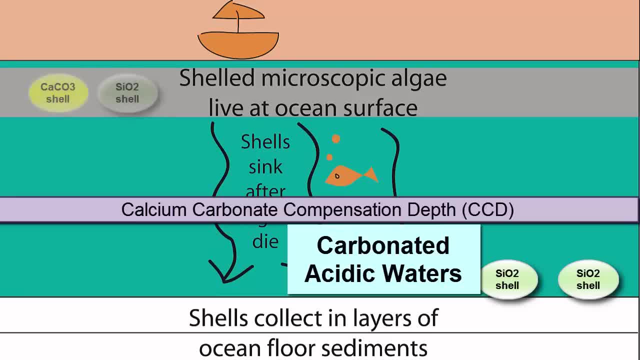 For now, we focus on the result. Though calcareous creatures might exist in the surface waters, their shells will dissolve en route to the seafloor. if the seafloor is deeper than the calcium carbonate compensation depth, Otherwise known as the CCD, 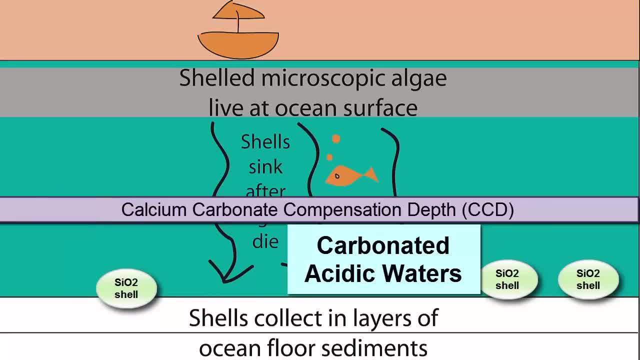 See you in the next video. The CCD is the depth at which the acidity of the seawater is high enough to dissolve these shells in their normal abundance, and thus no calcareous shells accumulate below this depth unless they collect faster than they can dissolve. 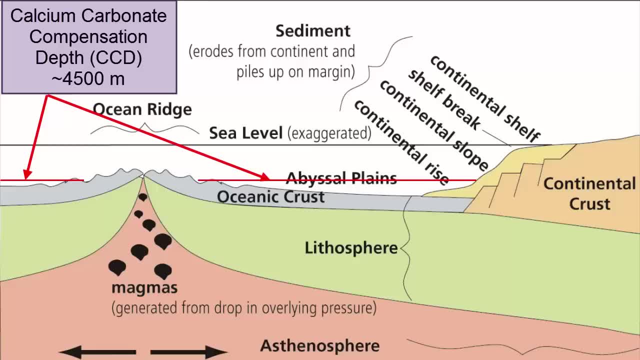 For our purposes, that means they should be absent. This depth varies in the oceans, but is on average around 4500 meters. That means the deep abyssal plains will not have calcareous shells accumulating. Only siliceous oozes or abyssal clays can collect at these depths.